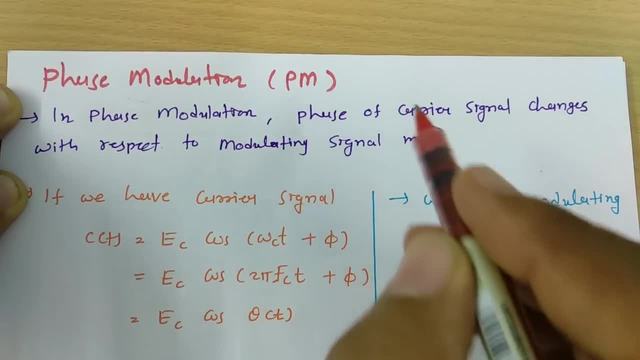 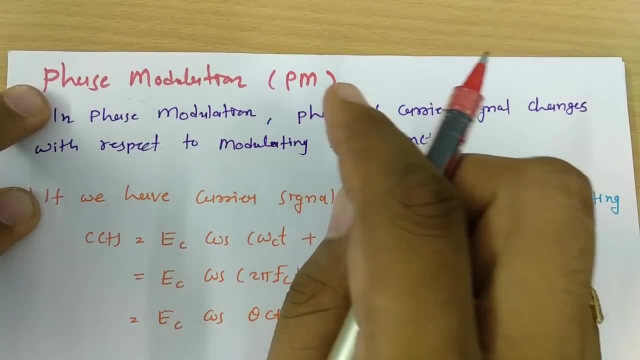 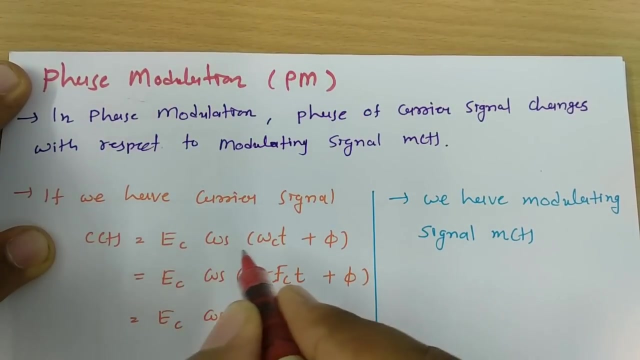 So when we talk about phase modulation, carrier signal's phase changes with respect to modulating signal. That is what phase modulation. Now see, if I say I have a carrier signal, that is this, which is what EC cos of omega, CT plus phi. So this is what the basic formula of carrier signal where in phase modulation we will be changing phase of. 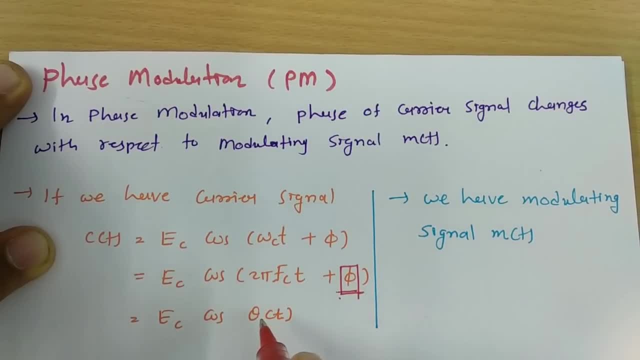 carrier signal. So if I say angle is theta t, that is this, then in phase modulation we'll be changing this phase with respect to modulating signal empty. So over here We will be changing phase five of carrier signal with return to modulating signal empty. 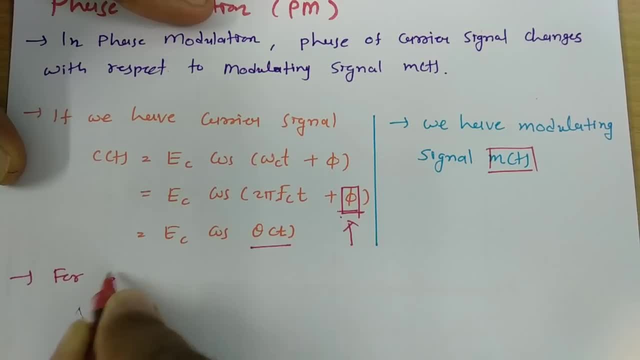 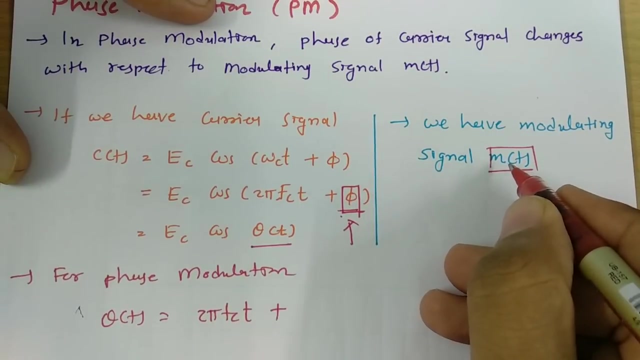 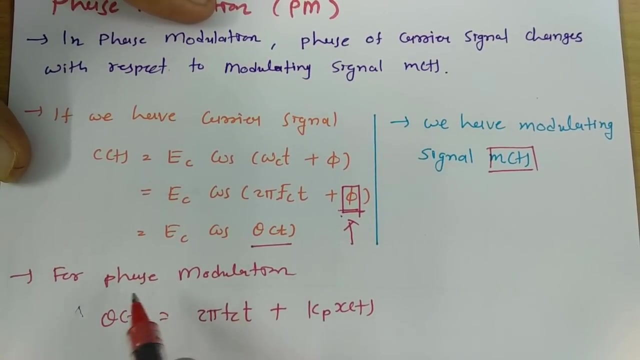 So for phase modulation we have theta t, that is what modified theta t with respect to modulation, and that will be 2 pi fc t plus that modified phase with respect to xt, that will be kp into xt. so that is what, basically phase modulation. so here, this is what angle and 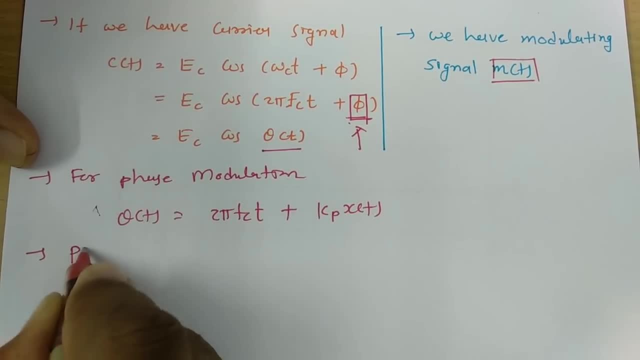 and wave pm, wave, that we can say. that will be. let us say y, pm of t. so that has to beec. where amplitude of carrier signal is not changing, that will be ec. so that has to beec. where amplitude of carrier signal is not changing, that will beec. 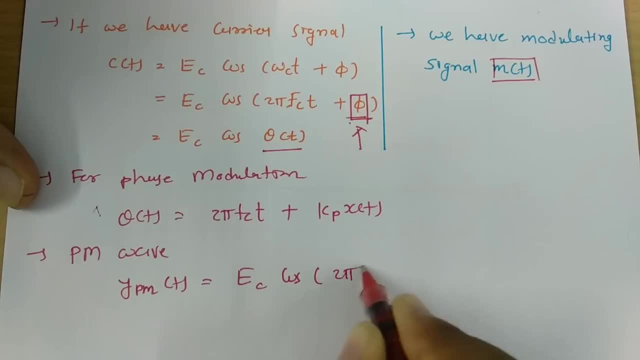 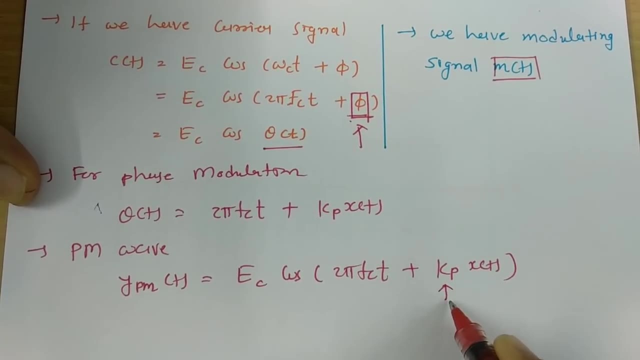 only cos of 2 pi, fc t plus kp, xt. now see over here this kp, that is phase sensitivity, vt and its unit, that is there in terms of radian per voltage. so what does this kp explains? kp explains us the quantity of phase deviation like see higher the value of kp sensitivity is. 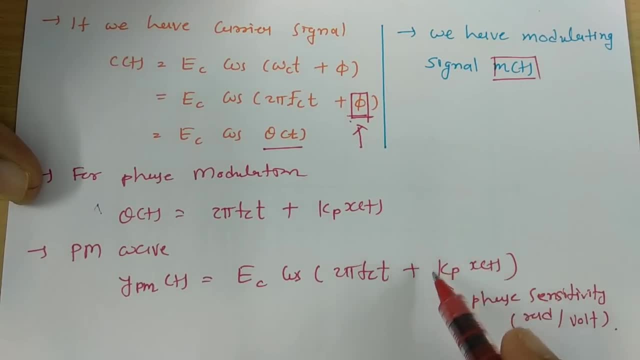 high. why? the reason is higher the value of kp, higher the value of phase deviation. so kp is what phase sensitivity? and here xt explains us whether phase deviation is positive or negative. like see, if i say xt is positive and x is negative, then it is positive and x is negative, and x is negative and x is positive. 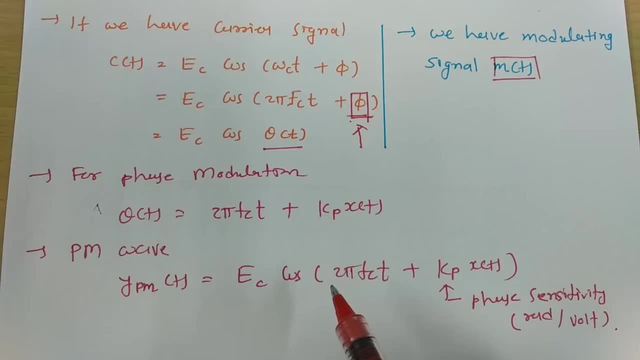 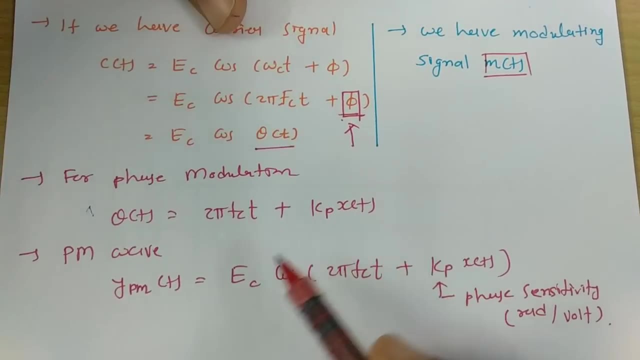 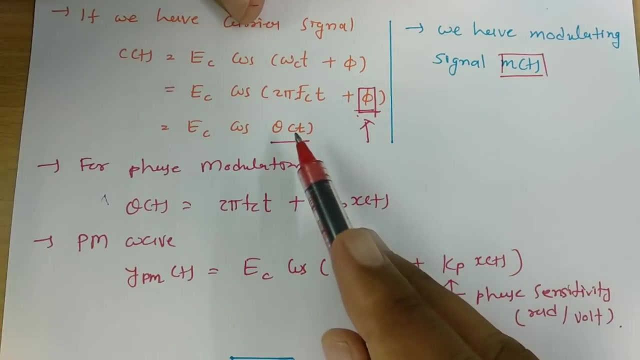 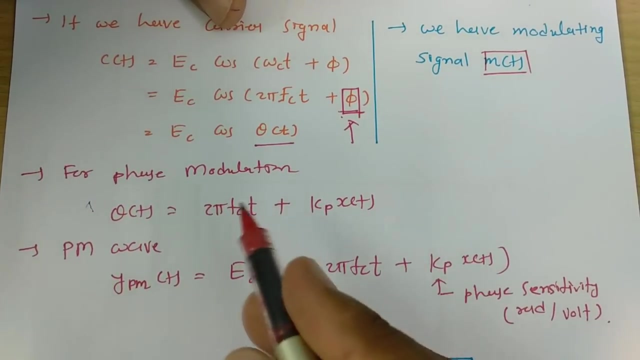 right now, then deviation of phase will be positive. and if deviation of phase is positive, we can say carrier will lag with respect to modulated signal. and if xt is negative, then deviation of phase is negative. it means carrier will lead with respect to modulated signal. so that is what we can say based on this deviation of phase. now, 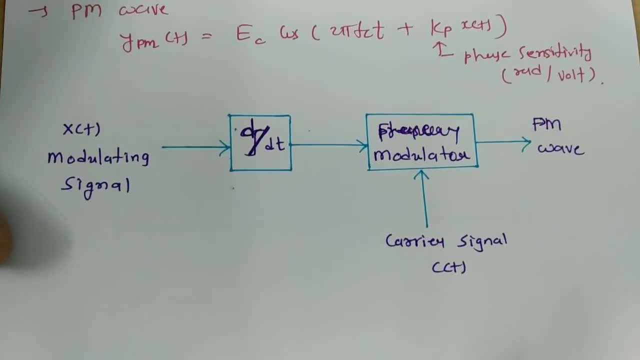 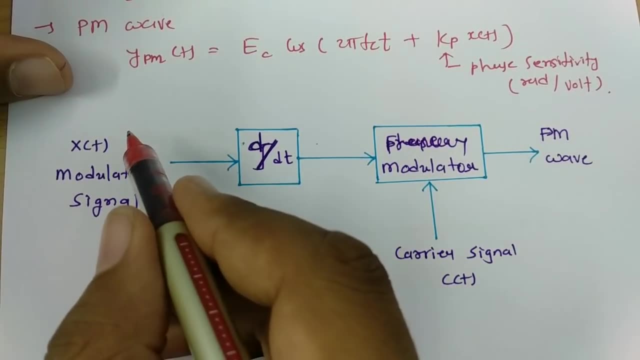 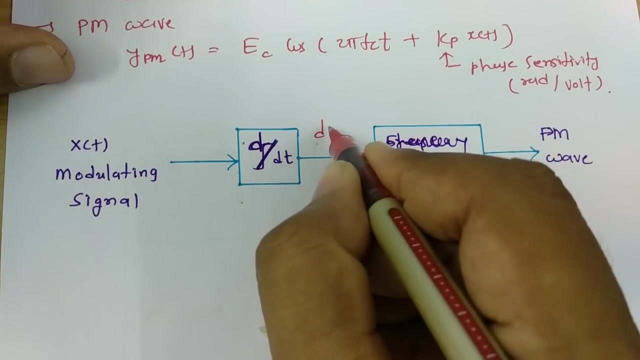 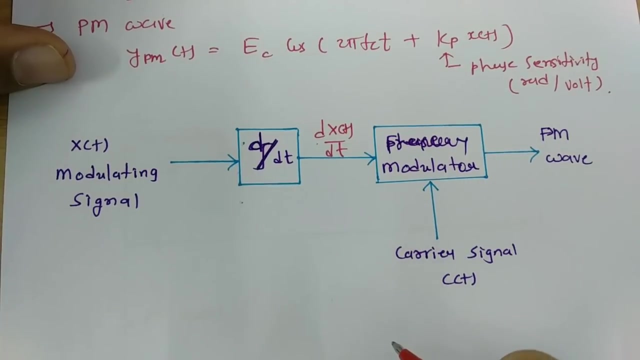 let us have phase modulator, how we can have phase modulation. so basically, what all we do is, if i say i have modulating signal and if i do differentiation, so over here i'll be having dx, t by dt, and over here i have a carrier signal and that carrier signal is ct. right, 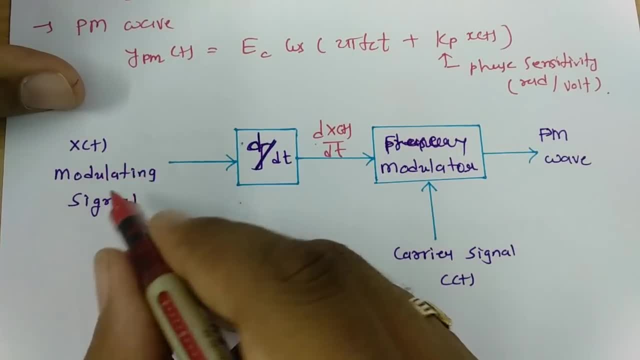 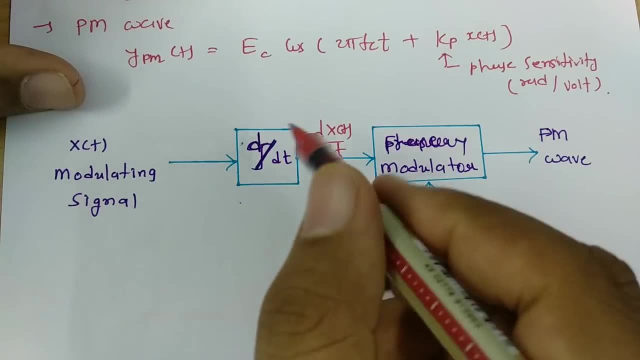 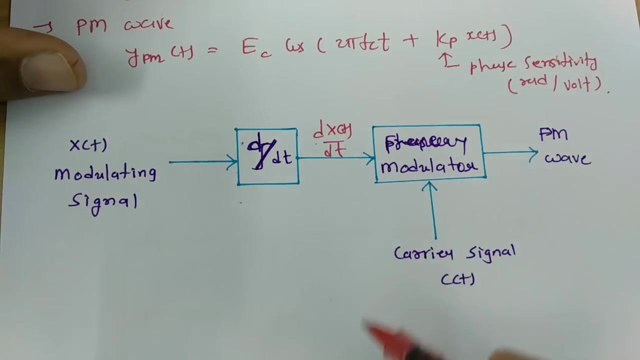 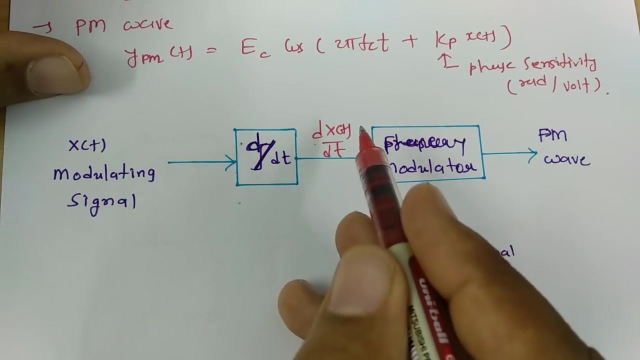 and over here we have that differentiated version of modulating signal. so this differentiated version on modulating signal, that is what we give to frequency modulator. so what does frequency modulator does frequency modulator that will add up an phase of carrier signal plus phase of. 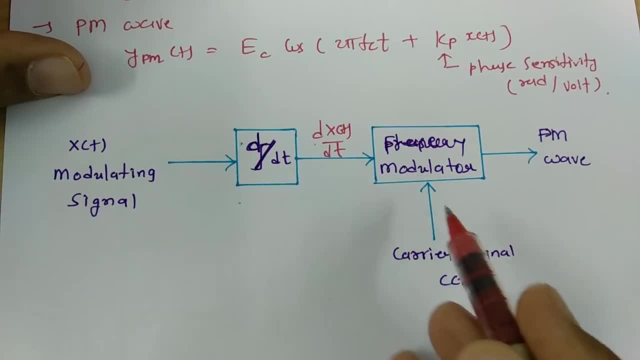 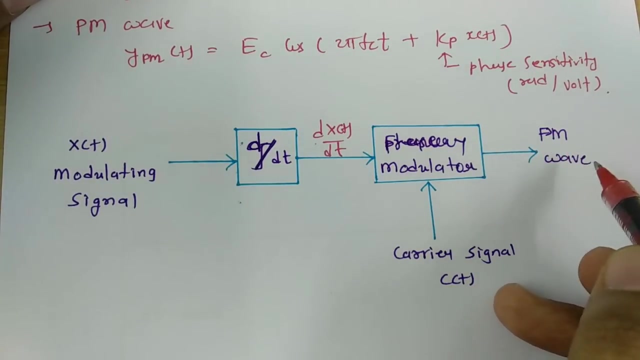 frequency. sorry, it will add frequency of carrier signal plus frequency of this differentiator. so if it adds frequency of both because of it is differentiator, differentiation of frequency results into phase. so that is what reciprocal process. so at the end you will be finding that is phase modulated wave over here. so frequency modulator. 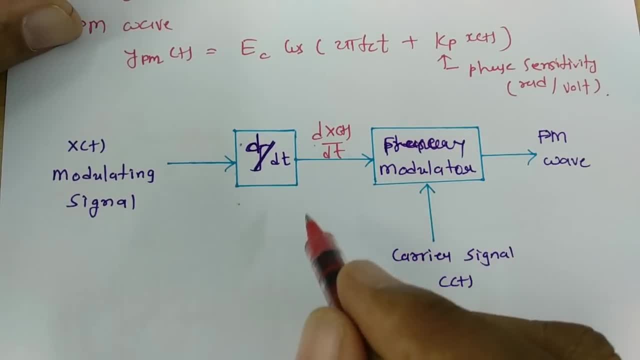 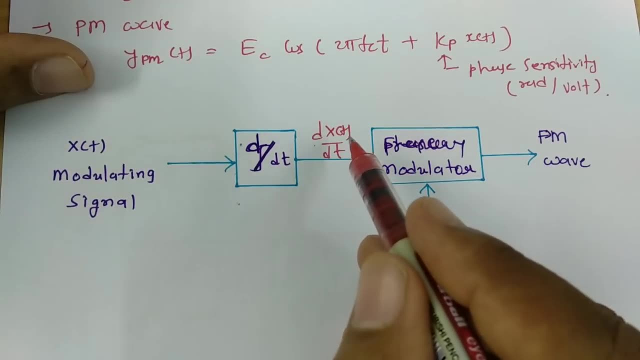 does what it will be modulating frequency. it means it will be adding these two frequencies. so here what I observe is this: is what differentiation of xt? so if it is differentiated version of that, it means it is what actually changing phase, and as if it is changing phase, then this is actually phase modulator. so this is how things are happening. 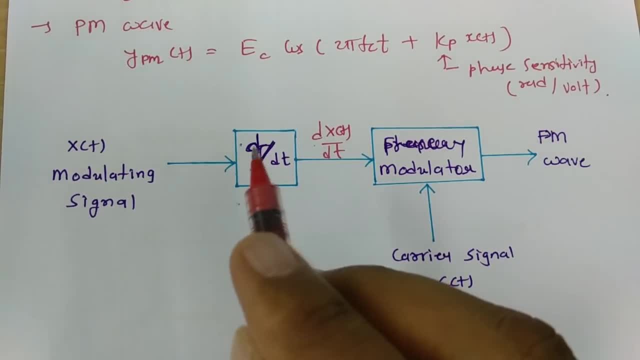 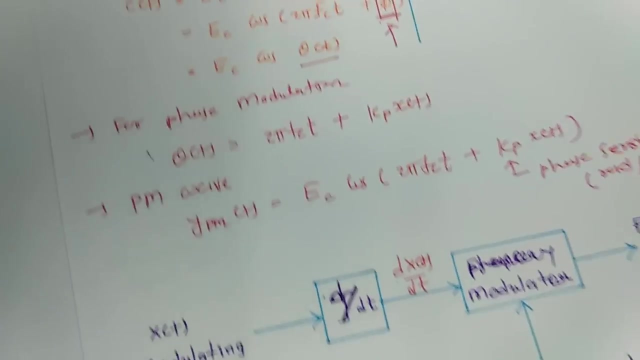 so ultimately, phase modulator can be made by passing that modulating signal through differentiator and then we can do frequency modulation of that signal with respect to carrier signal and we will be having phase modulated wave. okay, now let us try to understand waveforms of phase modulator, so it will be more. 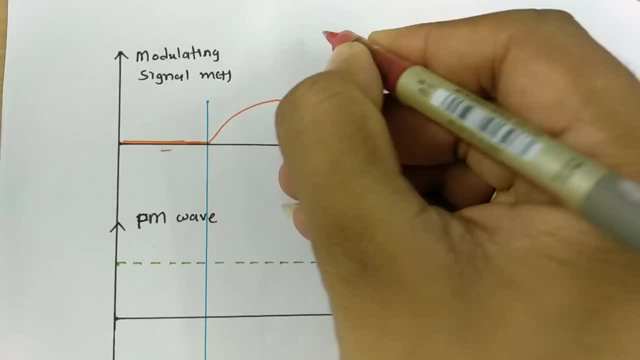 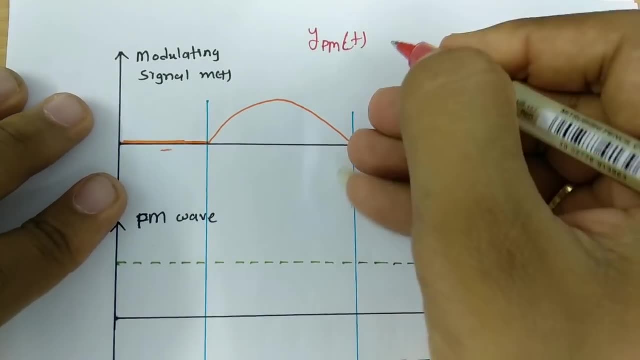 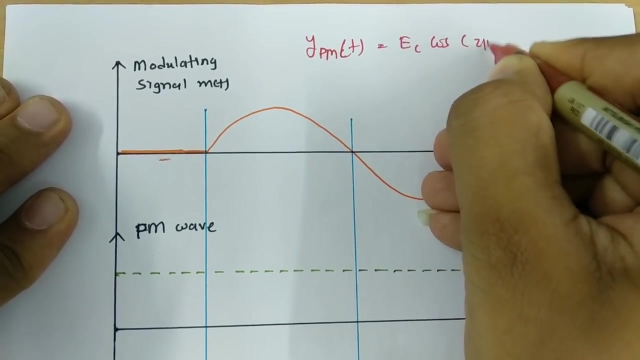 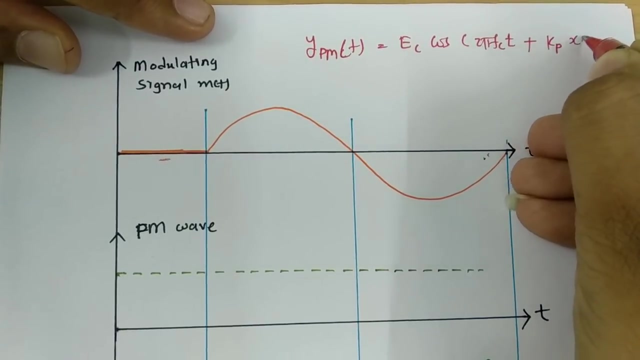 clear like see, as I have told you, waveform of phase modulator. that is, that is what we can have. it based on this basic equation that I have already told you right now: ac, cos plus kp into xt. now see over here: this is what deviation of phase. 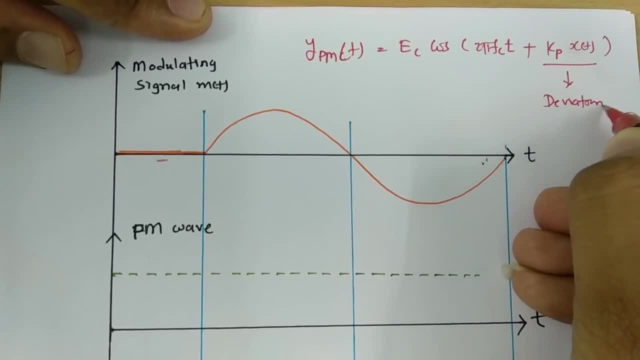 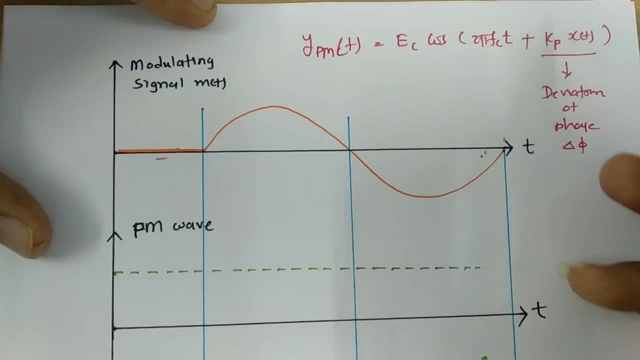 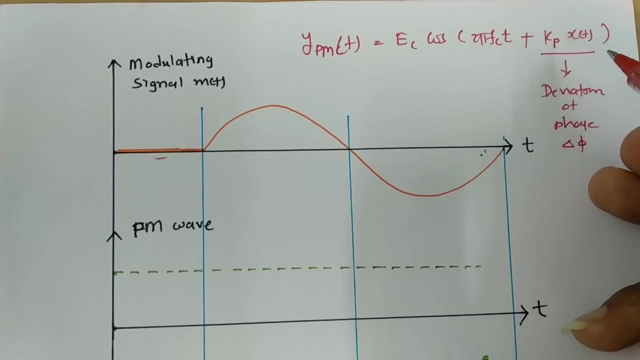 deviation of pap phase. let us say it is delta phi. So this deviation of phase that will be positive in case of modulating signal amplitude is positive and deviation of phase will be negative in case of modulating signal amplitude is negative and if modulating signal is positive, deviation is: 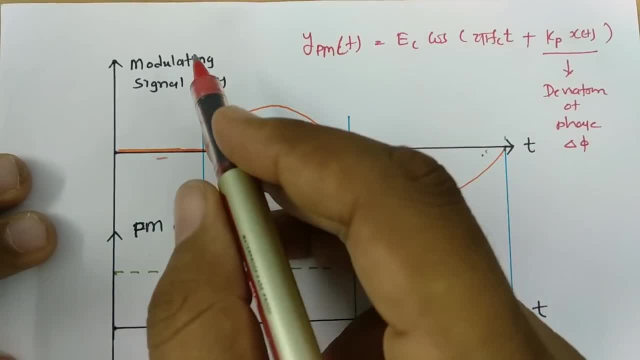 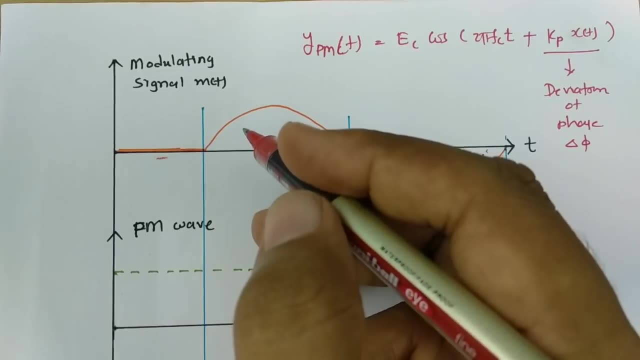 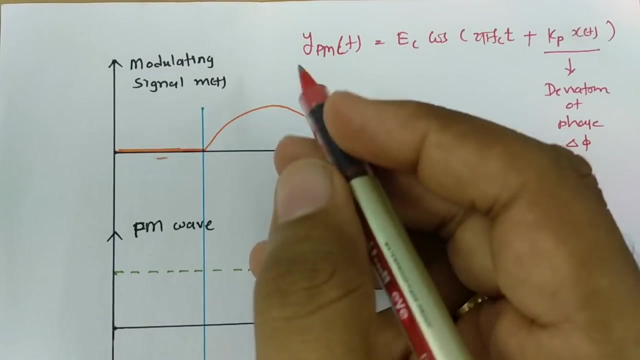 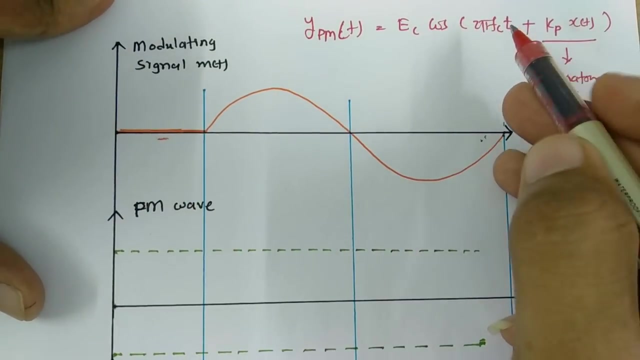 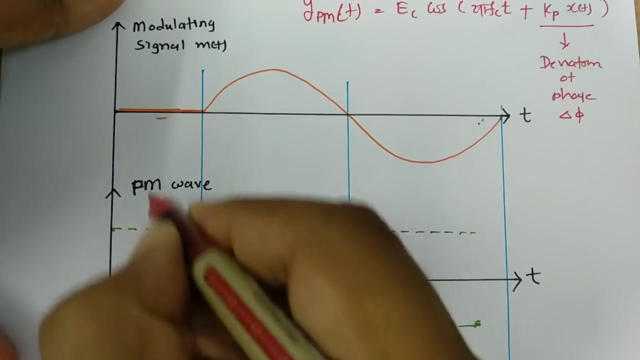 positive. it means modulated signal. that will be, that will be lag, that will be lead by carrier signal. means carrier signal will lag by modulated signal. Like see, if I say over here amplitude is zero, it means carrier signal is having zero phase deviation. So let us try to plot it: carrier signal will be having zero phase deviation, So 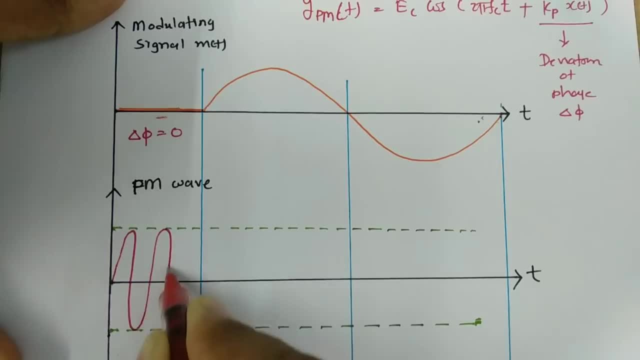 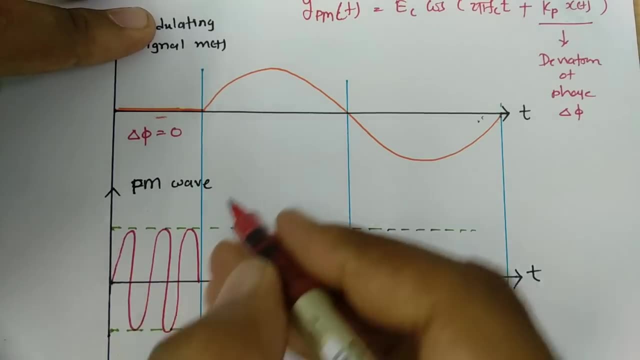 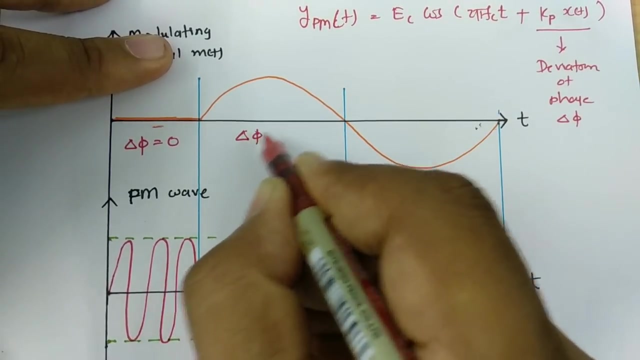 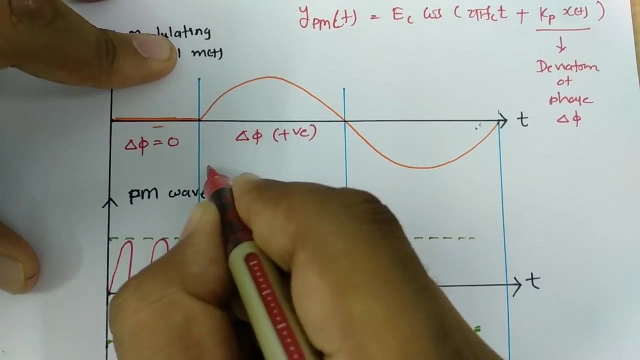 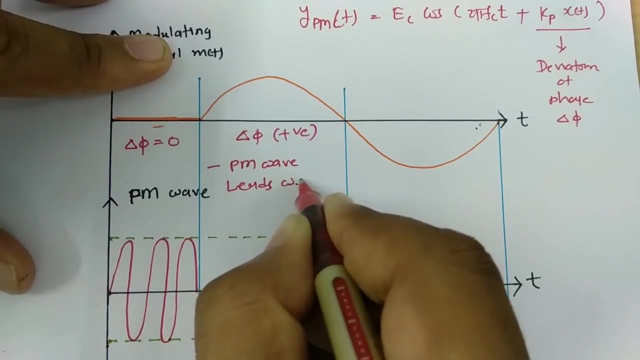 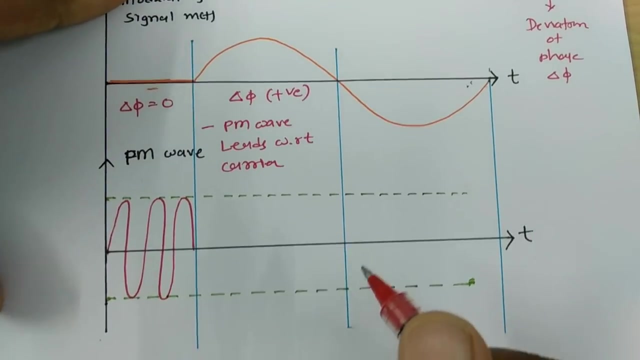 if I say this signal is like this: right, so there is no phase deviation right now, but over here, as as magnitude is positive phase deviation, that will be positive. So as if phase deviation is positive, we can say: PM wave leads with respect to carrier, or we can say carrier, or we can say carrier. 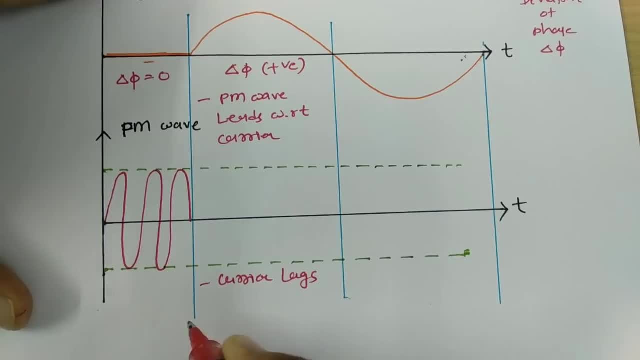 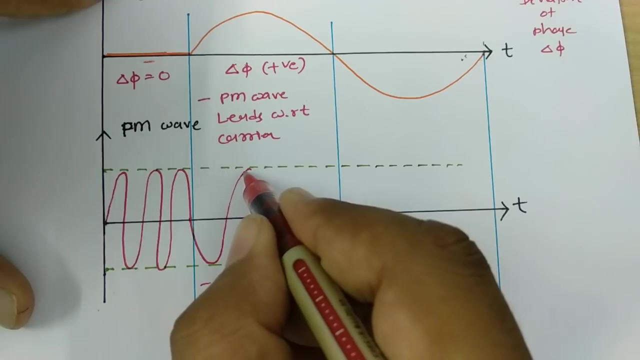 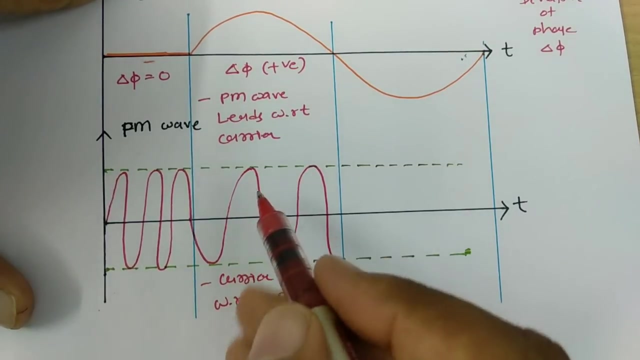 lags with respect to PM wave. So here, PM wave leads with respect to carrier. So if it leads with respect to carrier, you will be finding this wave is getting stretched in this direction. the reason is: now this wave should get lead. So you will be finding, see, it will be stretched like this right. So you will be finding. 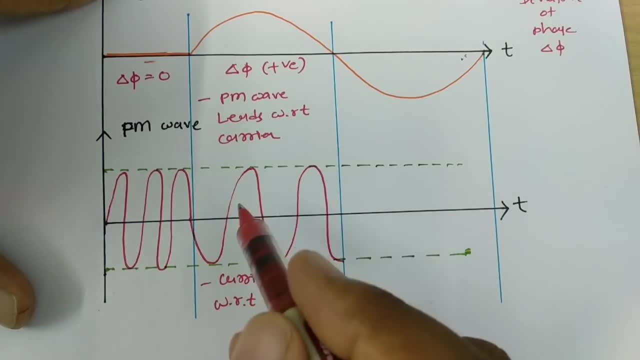 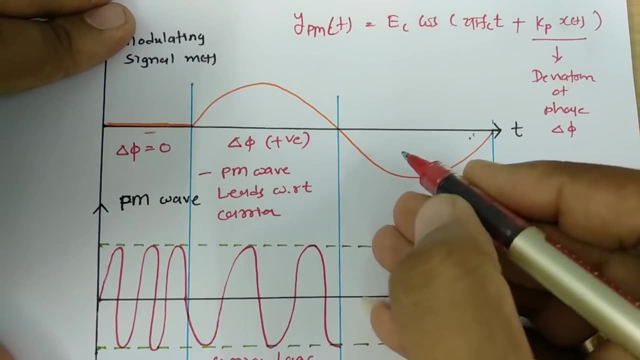 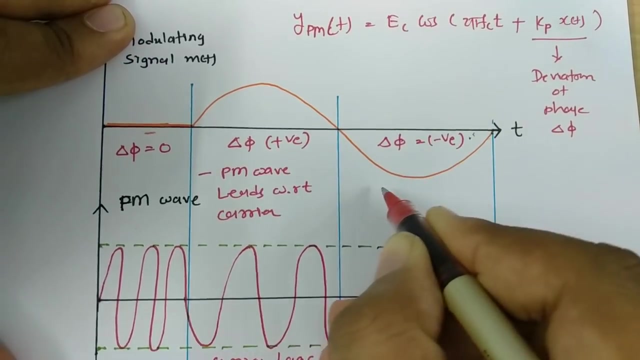 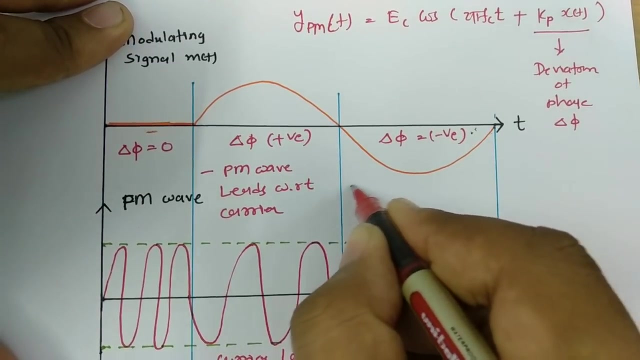 this is how PM wave phase that is getting lead with respect to carrier Now over here, modulating signal that is having negative magnitude. So as magnitude of modulating signal is negative, you'll be finding phase is negative. deviation of phase is negative. So if deviation of phase is negative, we 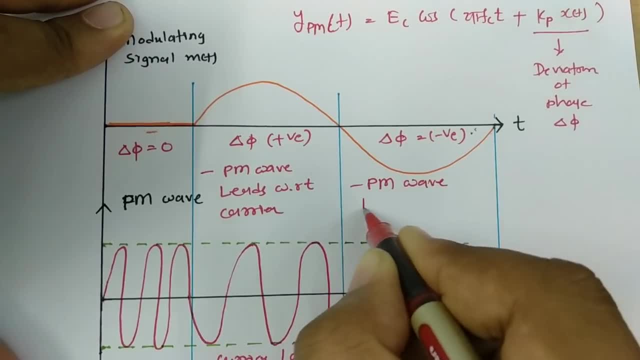 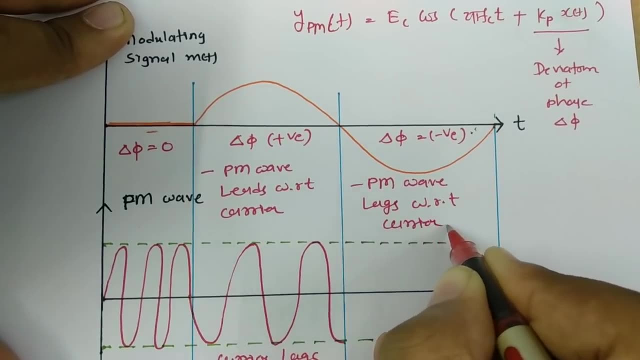 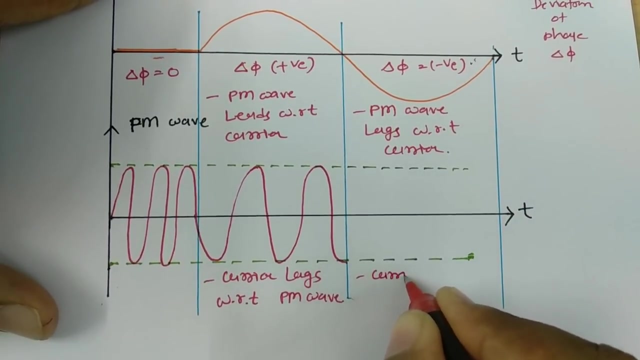 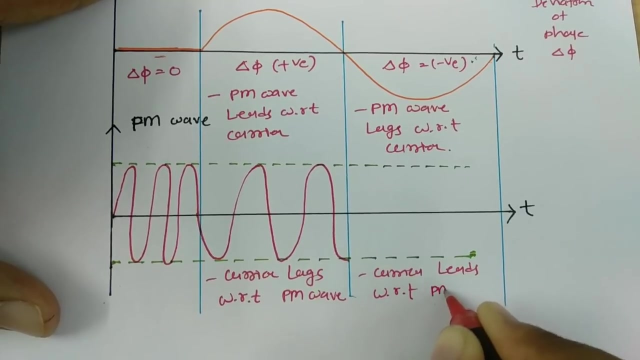 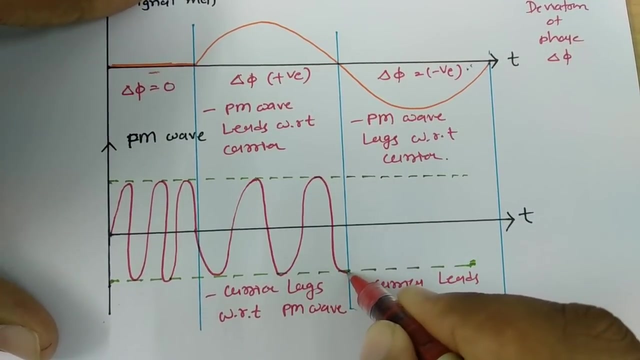 can say phase modulated wave, that should lags with respect to carrier. and if this phase modulated wave lags with respect to carrier, it means carrier leads with respect to PM wave. so what it means is now because of negative phase deviation. now you will be finding: 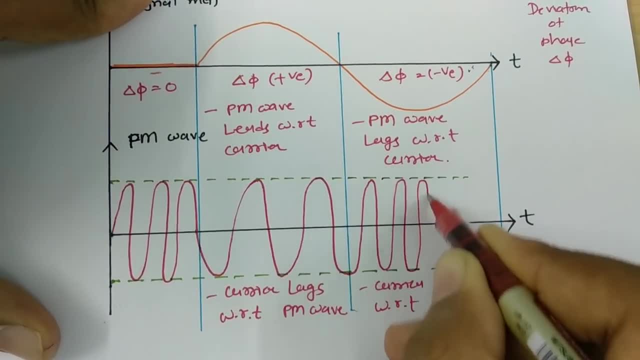 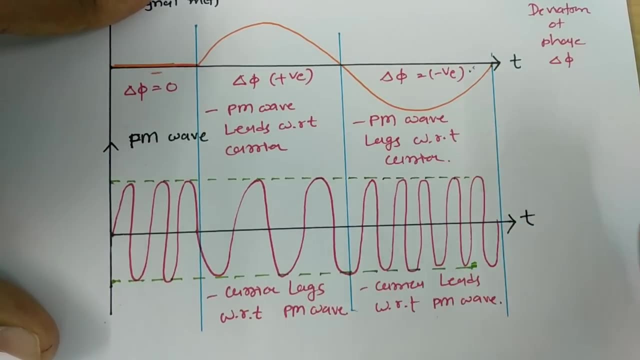 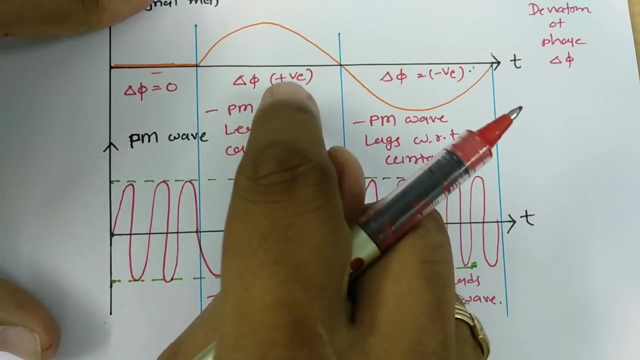 signal is very near to each other. so one can see over here frequency is increasing because of it is getting actually compressed because of lags of phase. so as a phase is getting lags, this wave is actually coming nearer to each other. and if phase is getting positive this way, that will get straight like this. so 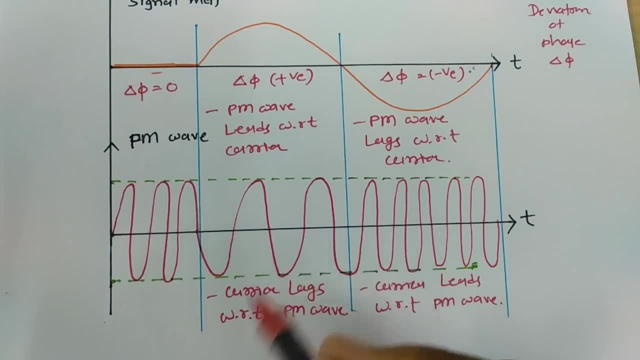 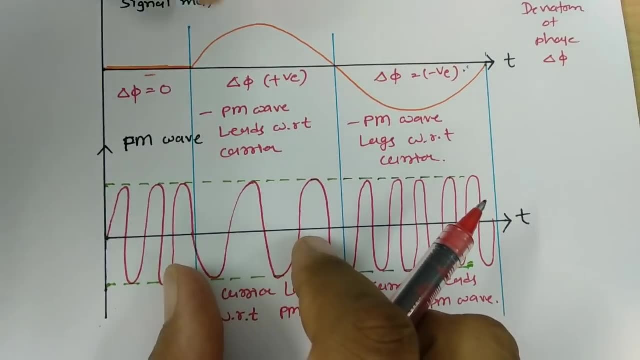 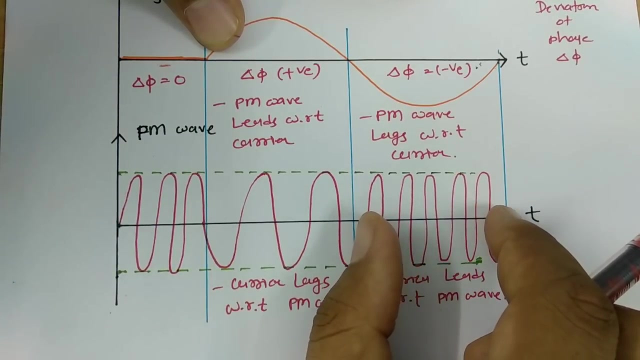 ultimately, this is what completely opposite to frequency modulation, where over here in frequency modulation you will be finding a- These cycles are very nearer to each other means frequency is increasing, and over here cycles are having more separation, so frequency is less over here in case of frequency modulation. 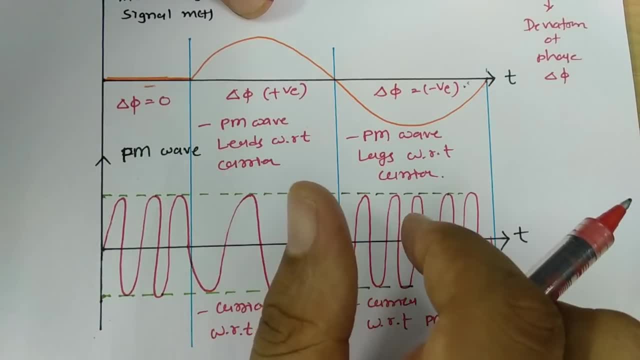 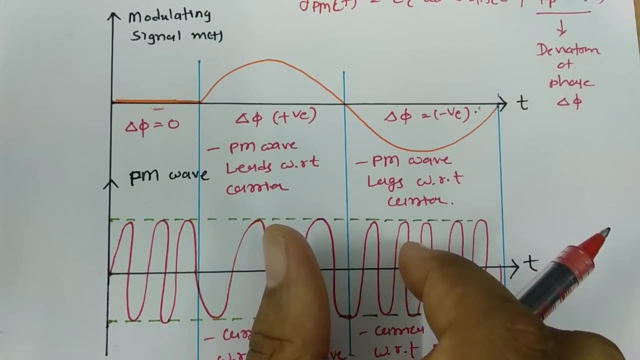 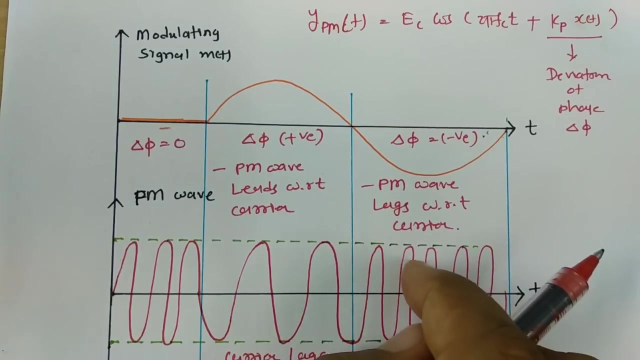 But in phase modulation this is quite opposite. So all we can say is by having just differentiation we can have that change. So very minor difference that is there in between frequency modulation and phase modulation. so that one should know Like in phase modulation we change phase. If phase deviation is positive, means phase modulated wave that will leads with respect to carrier means. 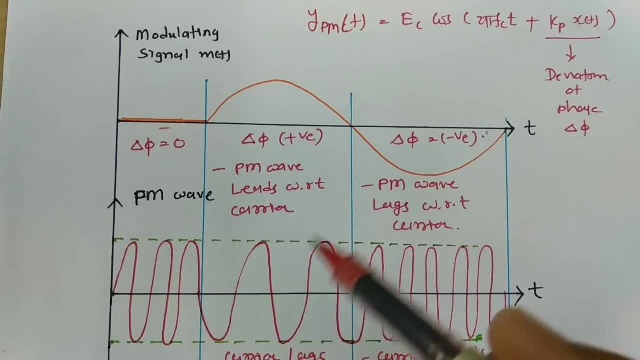 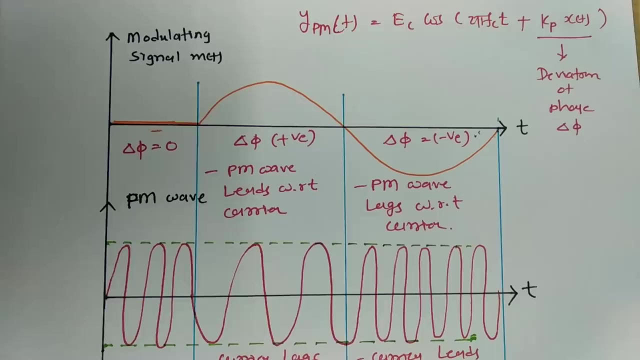 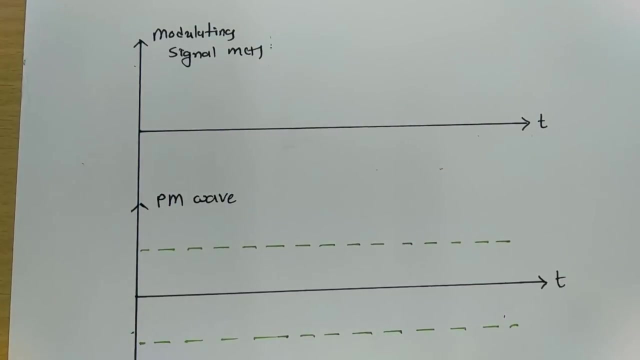 Now frequency will be low with respect to carrier, And if phase deviation is negative, means phase modulated wave lags with respect to carrier, means frequency is high. See, that is how case will happen. Now I will explain you second way in which what I will be doing is I will be considering square wave. 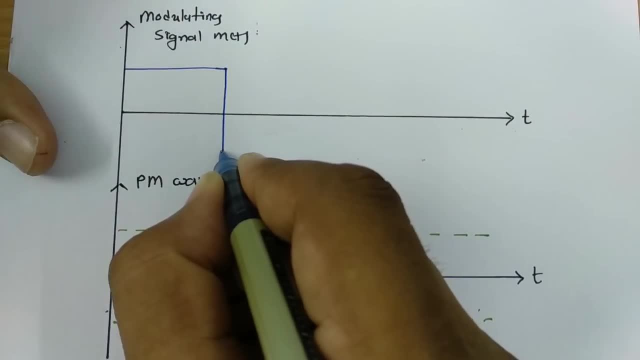 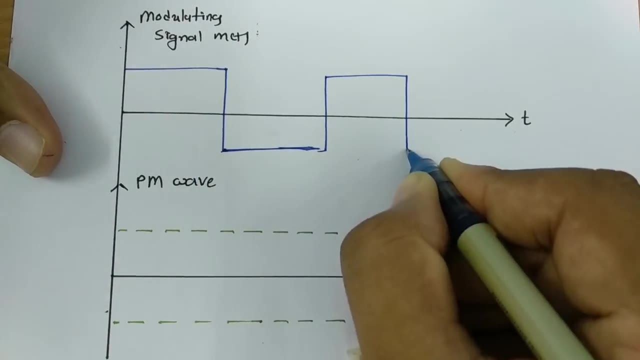 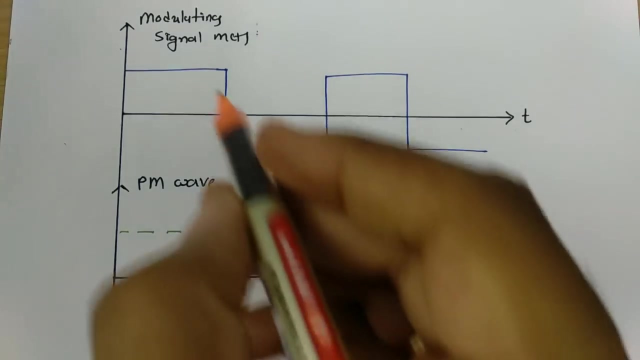 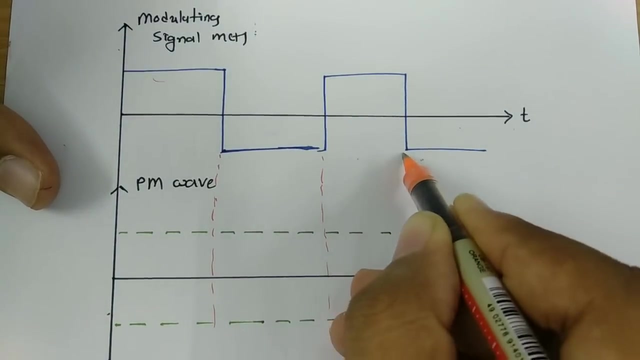 So if I consider square wave, So if I consider square wave over here like this, so I am just considering square wave right now, in this square wave here we have positive magnitude, and I am just stretching this trajectory to explain it properly. Now see, basically we have phase modulation. 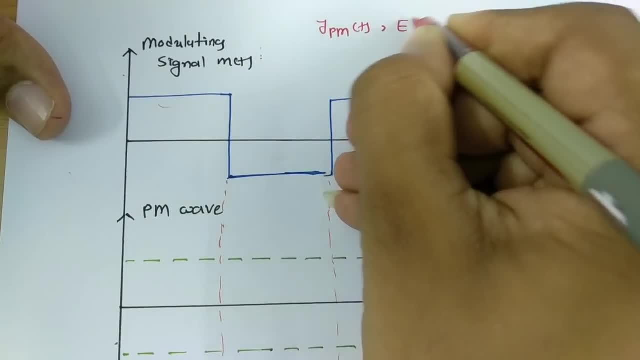 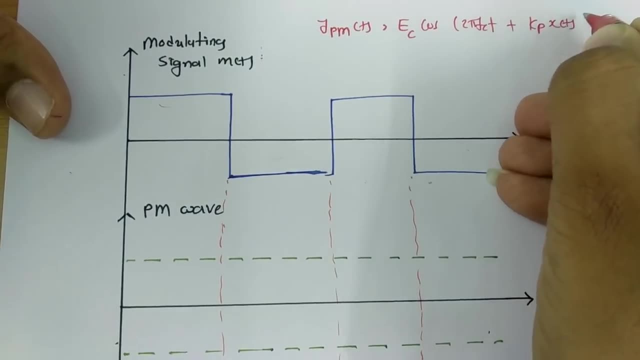 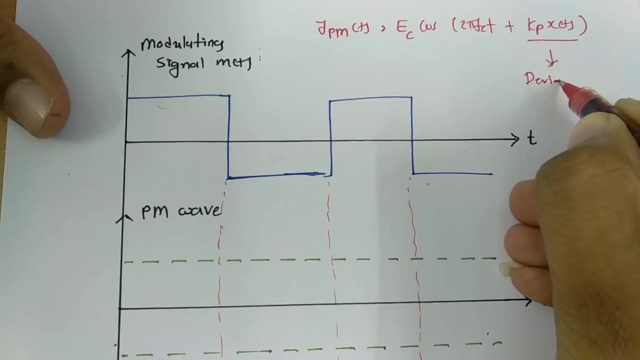 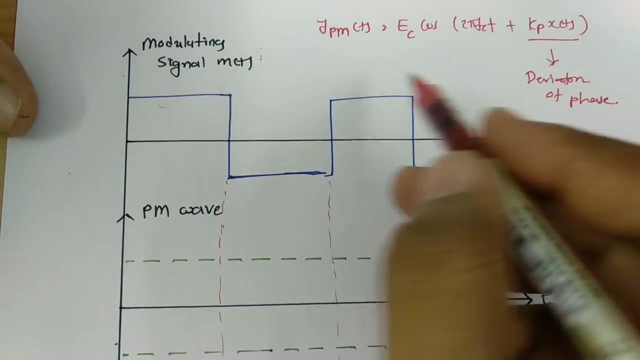 So this is phase modulation equation and that is EC cos of 2 pi fct plus kp xt. so we should remember this one where this is what, giving you idea about deviation of phase. Now what happens is in square wave till here we have positive magnitude. 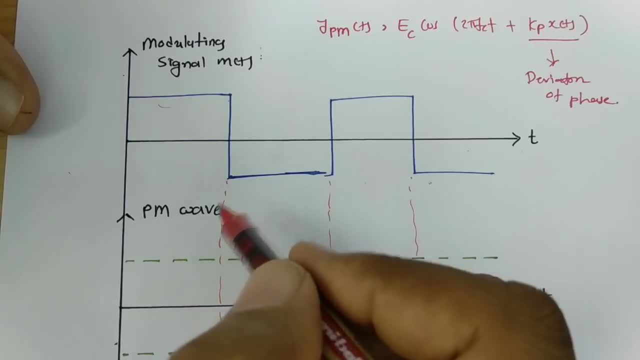 Now let us consider magnitude. Few times we are estimating magnitude And then we have given this: 4. This magnitude, so, as you know, it is the magnitude of the wave проблем. But what we actually do here, we we will be coming out with negative magnitude 때문에. In the same way, at this instant, we have positive with negative, therefore, and then after, suddenly, at this instant, we have negative amplitude and control. So for the second element, we have negative branded projects first. second point is due to which we will be redoing, obviously, particularUCK, which is reover happened. we will be indicating the value exactly. 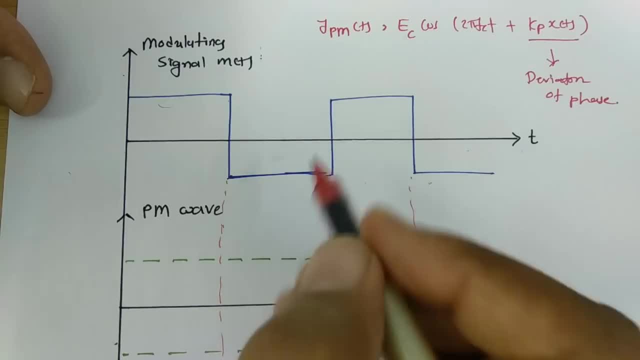 From here again there is complete reversal of phase, coming from negative amplitude to positive magnitude. right from here again there is complete reversal of phase coming from negative to positive magnitude. right from here again there is completely reversal of. right from here again there is people and what you get here, the reason is negative to positive magnitude. you will be quite 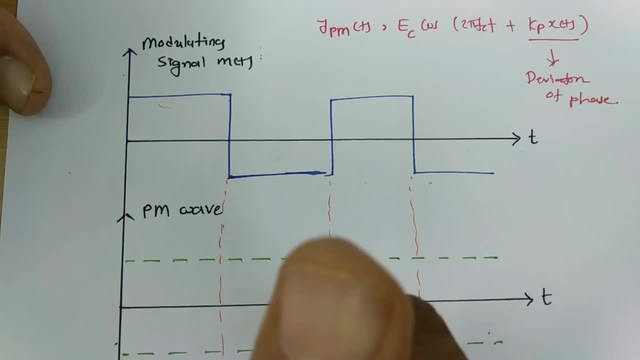 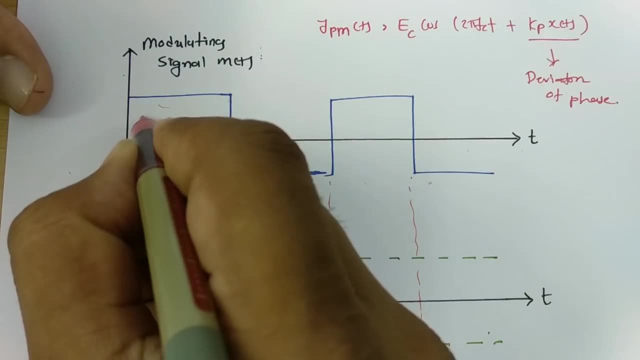 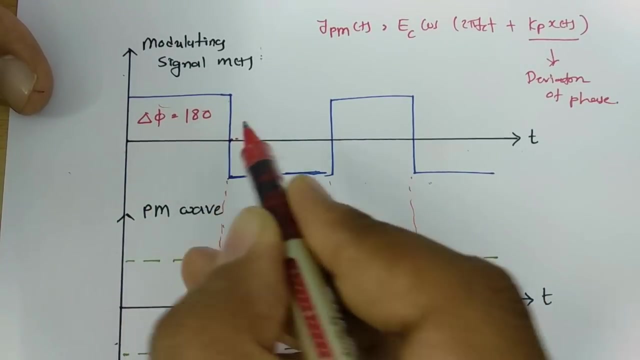 So so now what happens is a negative, positive magnitude. your professionals will be learning in phase modulation what happens over here. magnitude is positive, so i can say delta phi is 180, but as you come over here at this transition, suddenly delta phi that will get to minus 180. 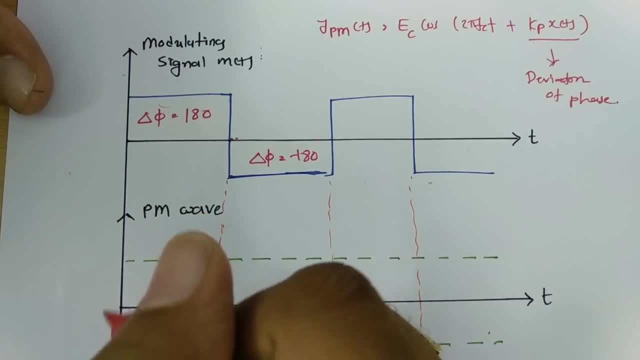 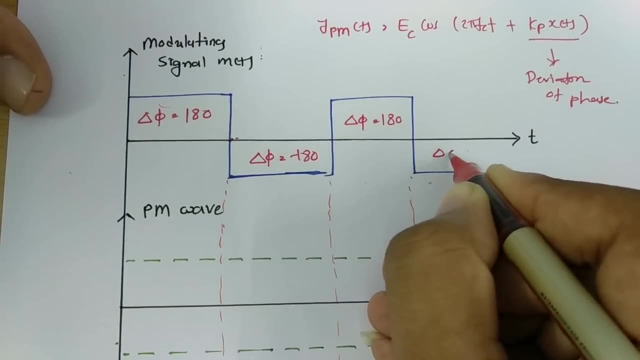 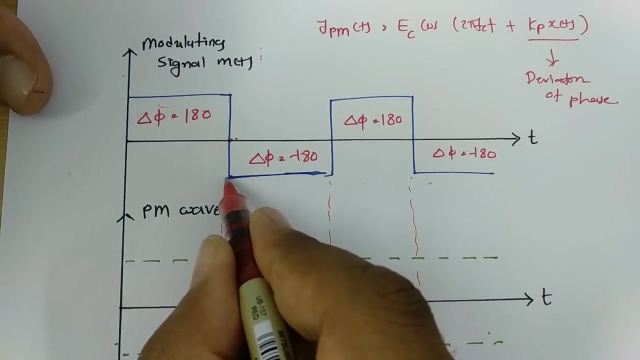 why. the reason is sudden change is there in deviation and over here, phase deviation is again plus 180 and over here again it gets to minus 180. so in square wave, what will happen is, at this instant, this trajectory that i have plotted, where you will be finding complete. 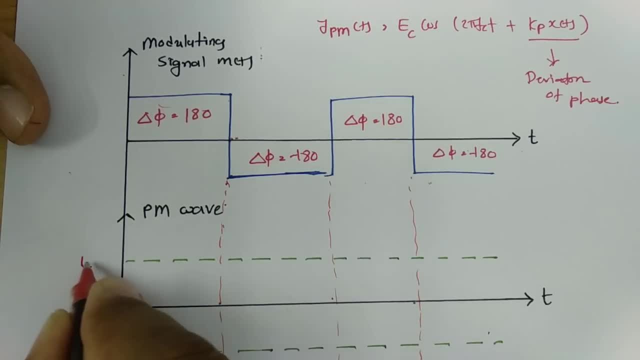 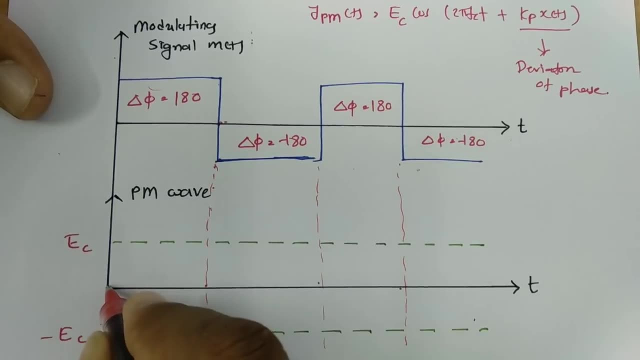 phase reversal is happening. so let us try to understand how it happens. i will plot it and try to explain you like how that phase reversal is happening. so see if i say signal is moving like this. so i will plot it and try to explain you like how that phase reversal is happening. 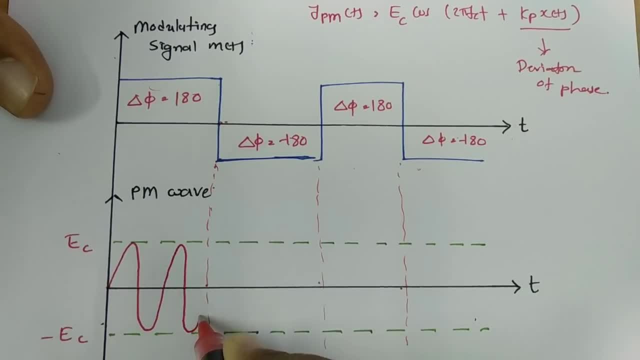 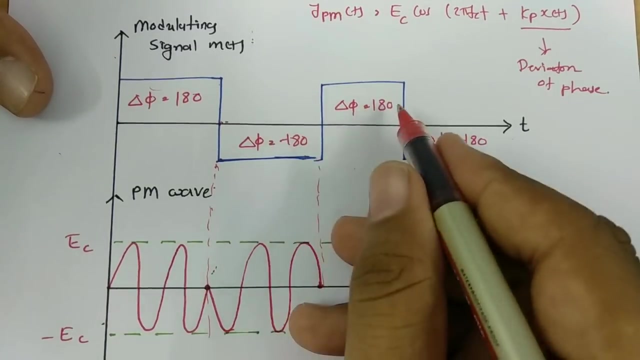 so see, if i say signal is moving like this, right, so when it comes over here there will be phase rehearsal. so now signal will flow like this: now it will not go in this direction, there will be phase reversal. so it will flow in this direction like this: now over here again there is phase reversal: minus 180 to plus 180. 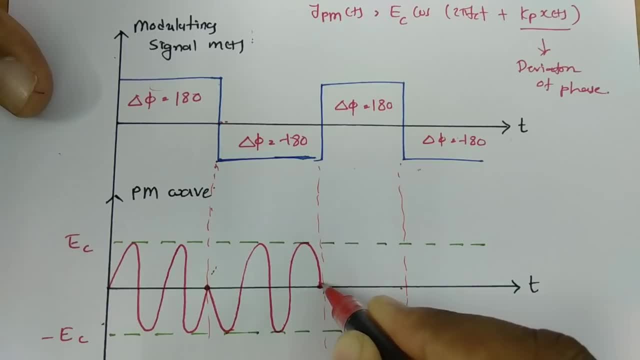 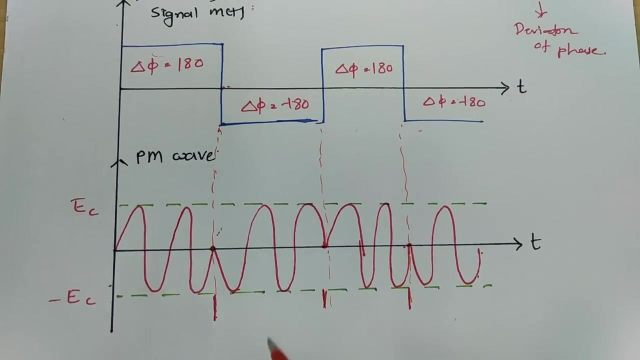 so signal will not flow in this direction now it will be having phase reversal and you will be finding it happens like this: now see again over here there is phase reversal. so again from here, frequency will be having phase reversal like this. so over here at this instance, right at this instance, you will be finding phase reversal are happening. so this: